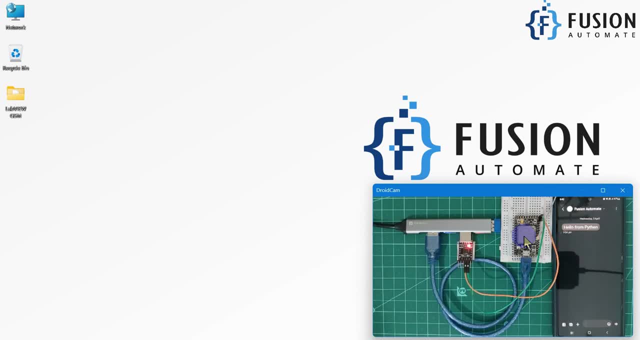 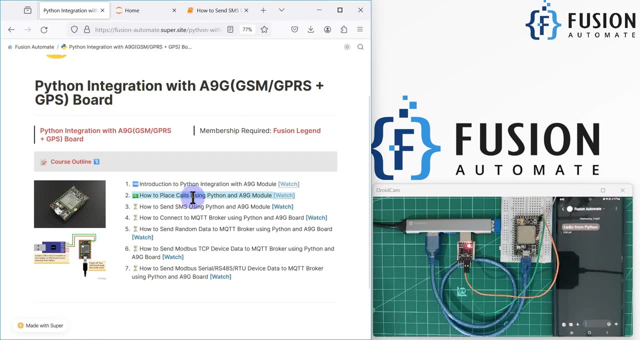 send the message body to that number and whatever number we will specify, it will send SMS to that number. So let's see how you can do that, and in the previous video we have covered this- how to place calls using Python and this A9G module. and in this video we will send SMS using Python and 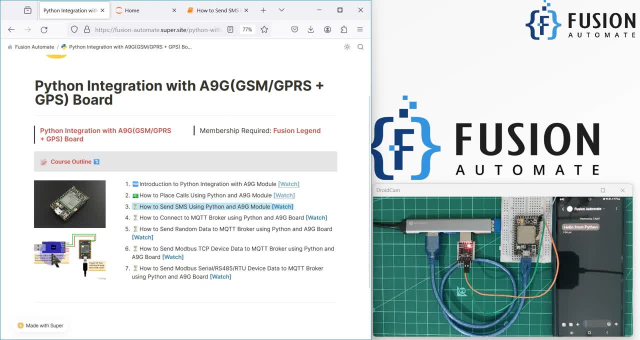 the A9G modules. Okay, so in this video we will send the SMS using Python and this A9G module module. if you want to see the connection diagram, okay, that how i have connected. you can refer this circuit diagram so how you can connect this cp 2102 module with the a9g board. okay, i have power. 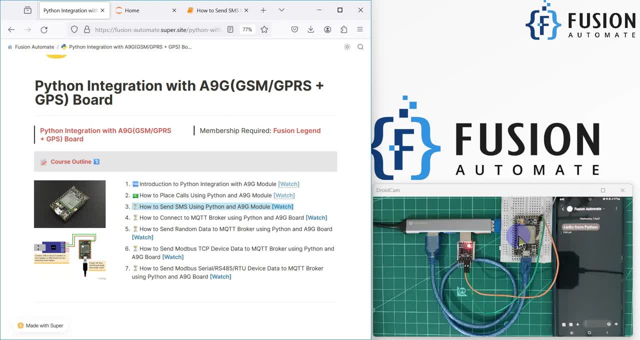 of this energy board using this blue micro usb cable and i am connecting this energy board with my system using this usb to serial converter. okay, and this energy board is connected serially with my laptop on the com5 port, so we are going to use com5 whenever we want to send the at command. 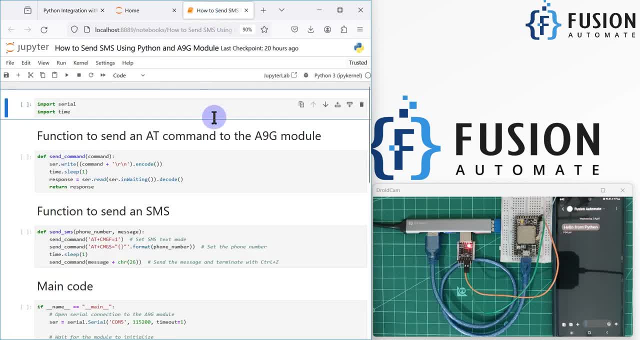 to this energy board. so let's see our python script. so here is the python script to send the at command. so let me reset kernel and let me clear all the output. okay, so first of all you have to import serial, because we are going to use the serial library to send the at commands. okay, and 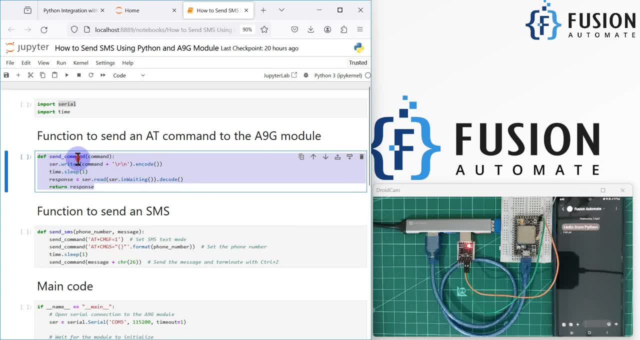 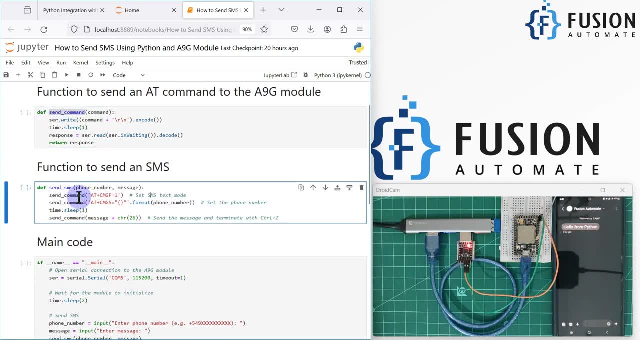 here is the default function which we have used previously. this will send at command to this a9g board. okay, so, function to send at command to the energy module. here is a function to create at command for the sms to be sent. okay, so first of all we have to. 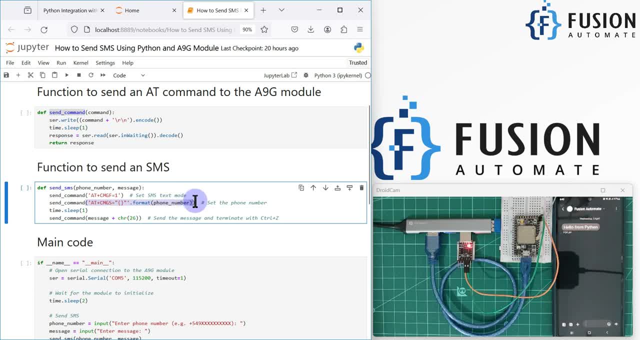 send this at command and then after we have to set the phone number and then after we have to add message. so this function will create the at command list for us and then, after it will send that at command to the energy board. you can see here: send command. so this function is using this. 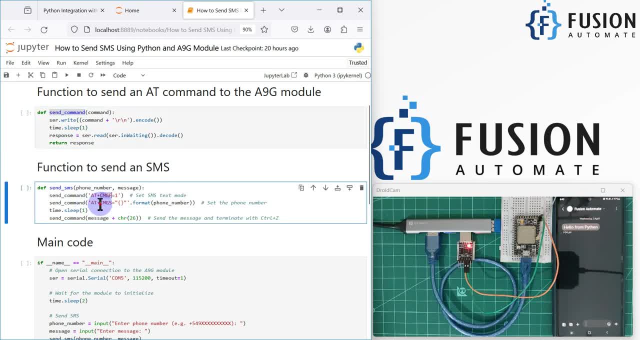 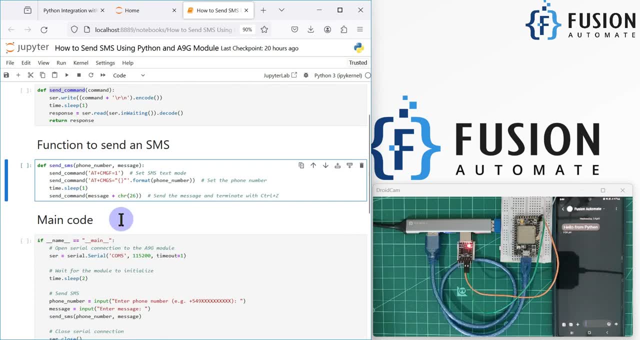 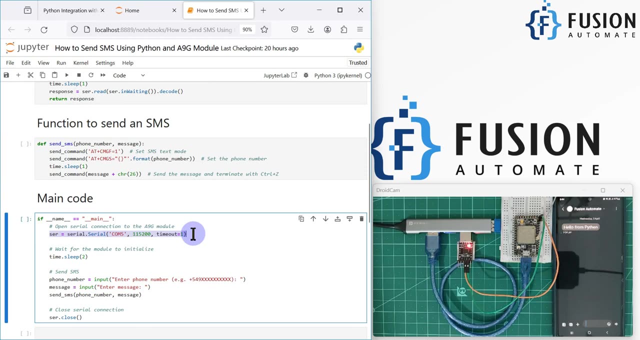 function okay. so first it will send this at command, and then after it phone number, and then after it will send message. okay, what we want to send, and this is the main code which is used to execute these two functions. so first of all, we are creating serial object to 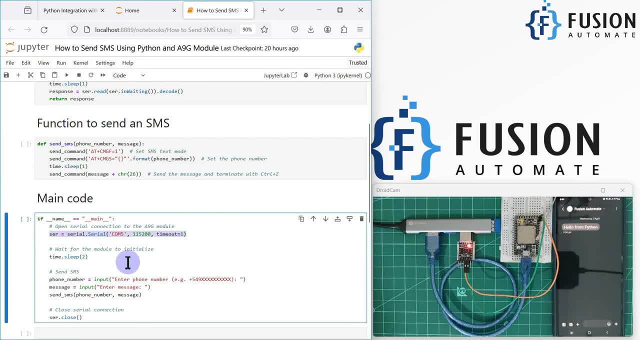 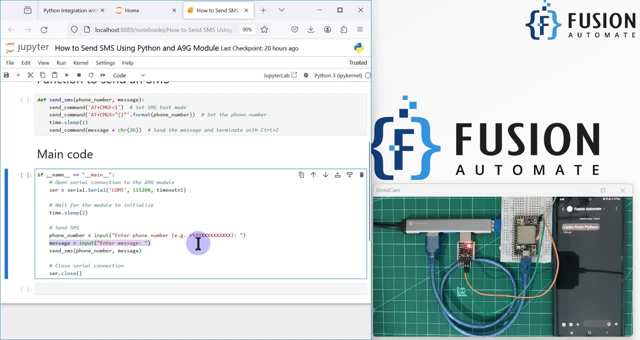 open the connection between python and this ing module and then after we will ask user to enter the phone number with country code and then after again, we will ask user to enter the message body, and once user enter the message body and once user hit the enter button, it will execute this. 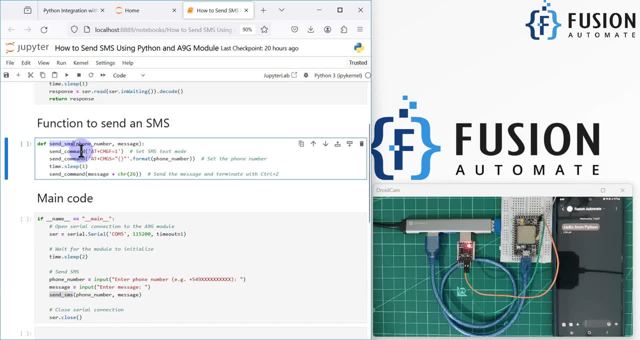 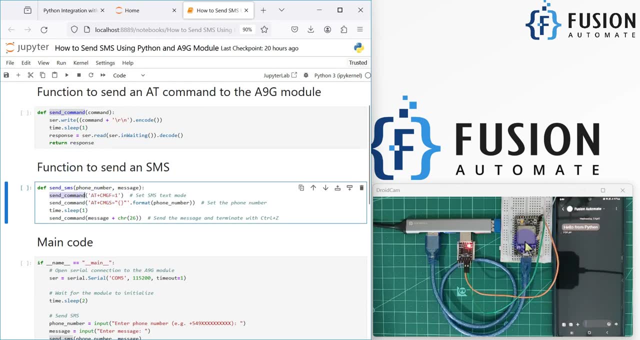 send sms function. and send sms function will execute this command first, so it will send this command to this ing module, so sms mode will be set to text, and then, after it will send phone number. so where you have to deliver the message that will be specified here in this command and what. 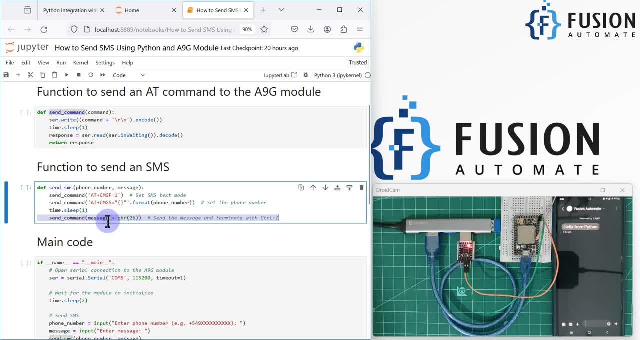 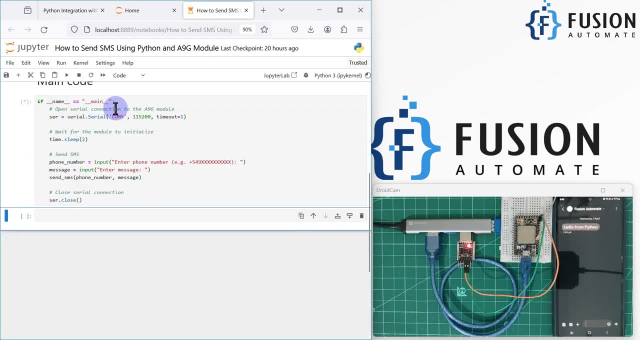 message you have to be delivered that will specify in this command. okay, so let's execute all the cell one by one. okay, and here is our main code. so it will ask for a phone number first. so i'm going to provide my number plus 91, okay, and i'm going to hit enter and then, after it will ask for the message body which we want to. 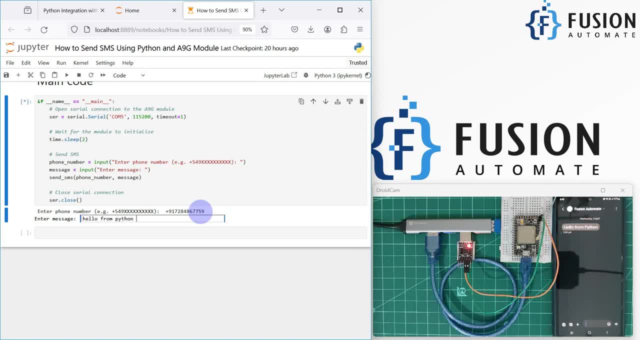 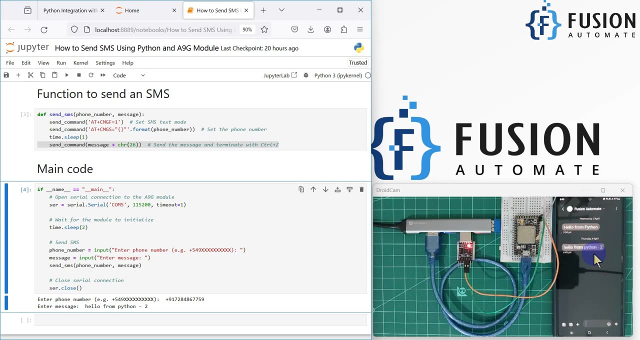 send. so hello from python. and this is the second message. so i'm going to hit enter and once i hit enter, it will process it. it will send all the at command one by one and after successful execution you can see we have received the sms. okay, i can rerun this main code again. it will again ask for the. 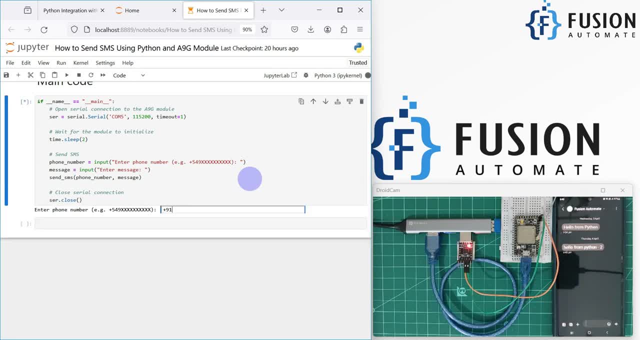 phone number so i can provide same number. otherwise, yeah, same number and i can type the message: hello from python and we are going to do the third test. so i'm going to use three and hit enter. the message will be delivered here. okay, you can see we have a message, so this you can use whenever you want to send any alert sms. 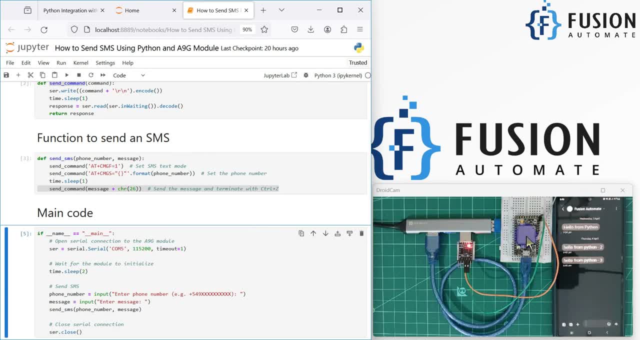 okay, this nng board also work with the gps. so in the emergency, if you want to send the gps location via message, then you can use this functionality. okay, so it will first fetch the gps location and then, after it, will send the gps location. so that's it. so now let's see how it works. so if you go to the 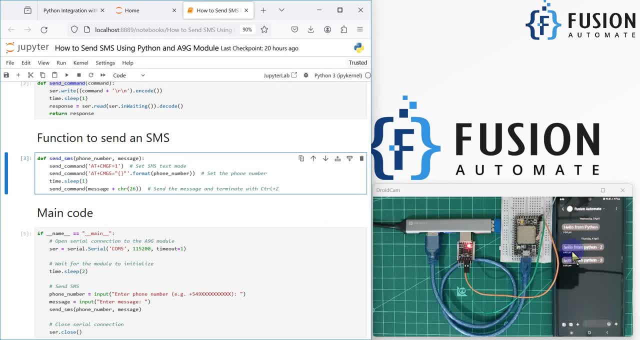 will send the GPS location via SMS. also, we can use in some alert system whenever our critical parameter goes beyond some certain limits. okay, so we can also include the value of that parameter in the message as well. so there is unlimited possibility with the SMS. okay, whatever you want to do with the SMS. 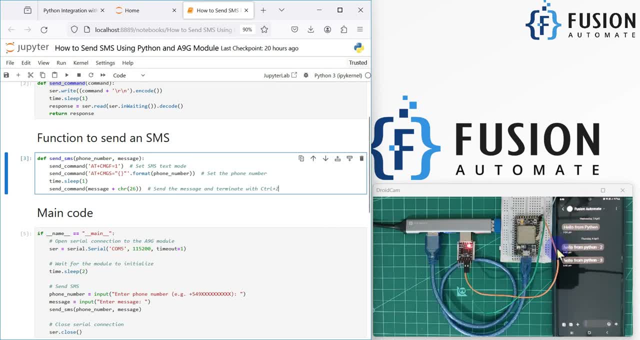 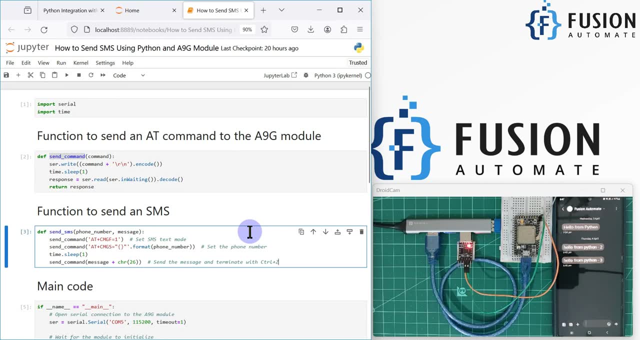 automation and Python. you can do it here. so it's up to you how you want to design it, how you want to program it and how you want to implement it. okay, so this is all about how to send SMS using Python and the NIG module. so you have to. 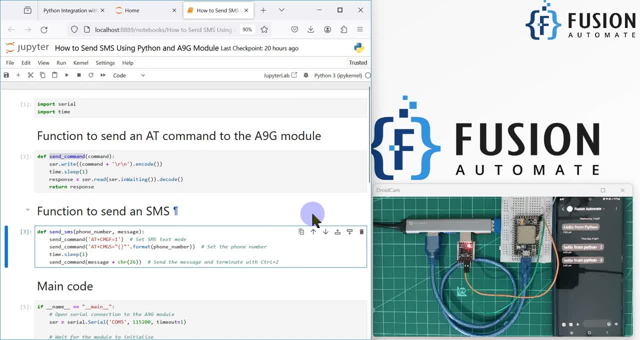 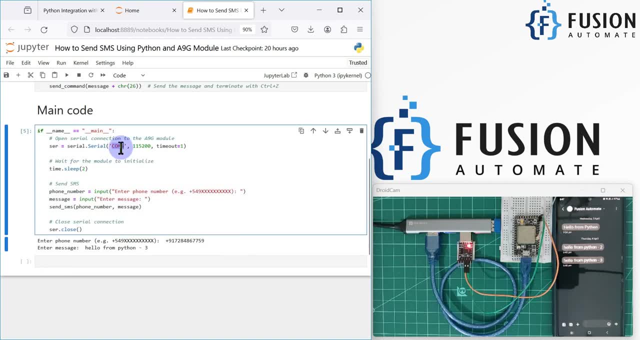 connect your NIG module with your Raspberry Pi or with your Windows operating system or with your Linux operating system. you can use this Python script: just change the baud rate, com port and everything based on your system. if you are using Linux, then this you know- port definition will be different. 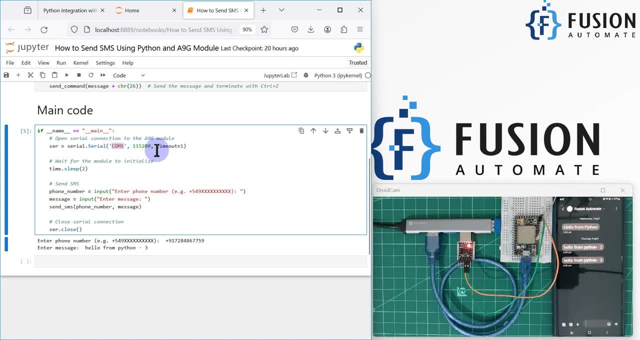 so you have to correct this port definition in the Linux and Raspberry Pi. in the Windows you will see like com5, com2, com1, okay. so that's it. and if you want to fix it, okay. if you want to fix the phone number and the message, then also you can do it. so if 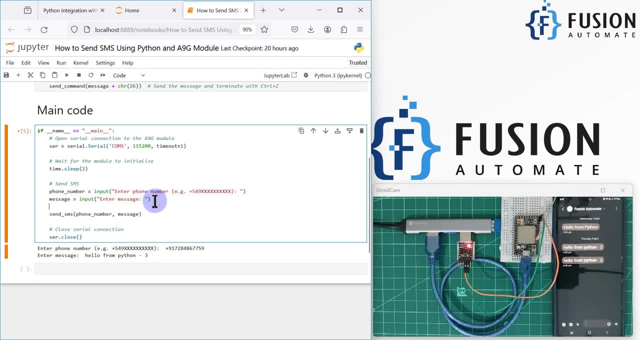 you want to fix it, then you just have to use like this: so we are going to fix the phone number and we are going to fix the messages. so you can fix phone number by typing here: so plus 91, okay, and I'm going to fix my message. I mean message. 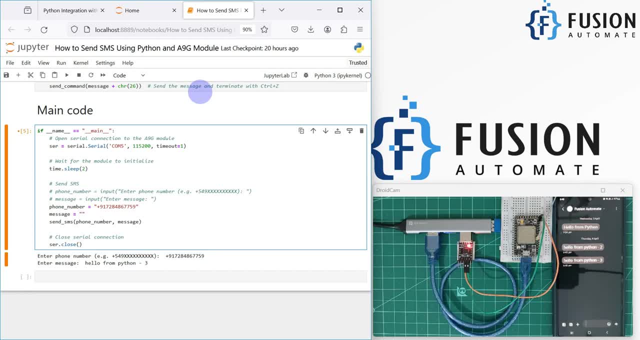 body using this. so what you want to write, you can write here. okay, I can write multiple lines: line 1, line 2, line 3- from Python, okay, and I can run this code and the message will be delivered to my number. you, qui, you can see line one, line two, sorry, line two- two times, and from Python, okay, 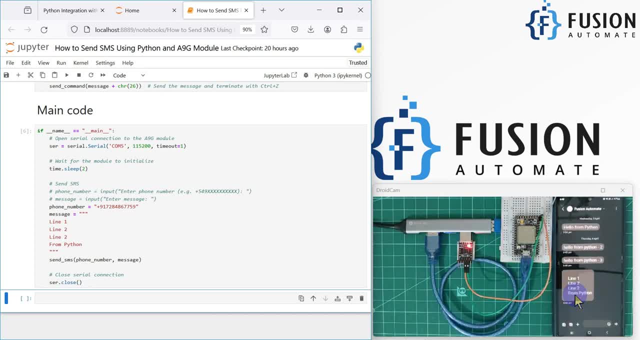 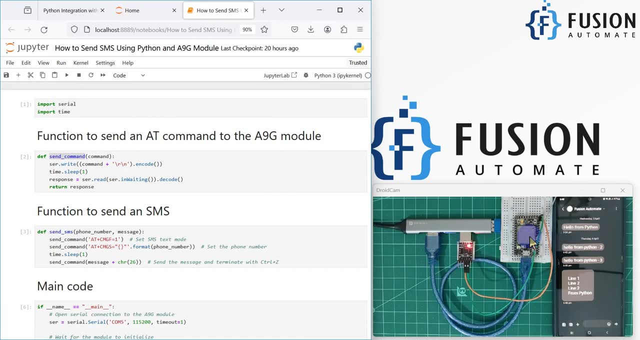 so this is how your message will be delivered to any number. okay, and this is how you can use Python and this, a 9g module, to sign the SMS. also, you can receive the SMS, but that portion we we'll see in the future videos. you can. 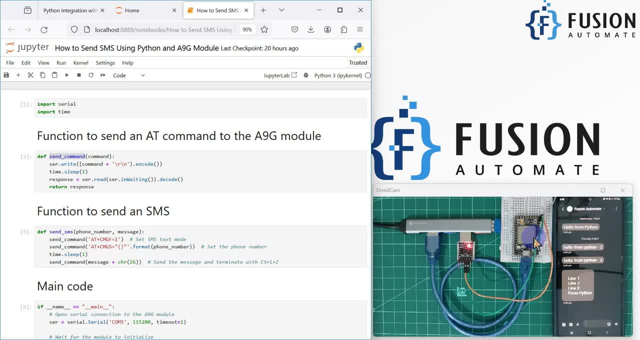 receive the SMS. you can, you know, extract some particular word from the SMS and, based on that, what you can process, something you can turn off, something you send email, whatever you want to do you can do based on those, uh, specific words. okay, so that is also possible with the anng module and the python programming, and you can also use the script. 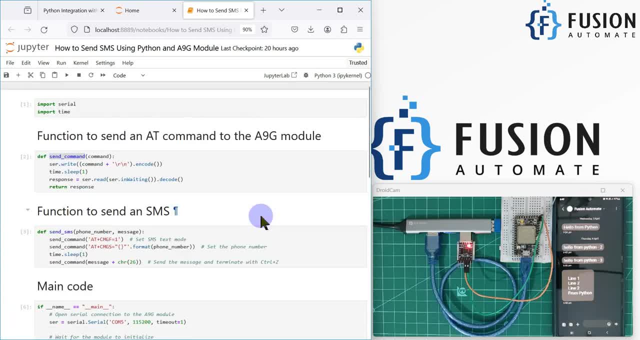 in the raspberry pi so you can use it anywhere, wherever you like, okay, so i hope this thing is clear, and if you still have any question or any doubt, then you can always ping me on telegram, instagram, whatsapp, and in the next video we are going to see how you can use anng module to